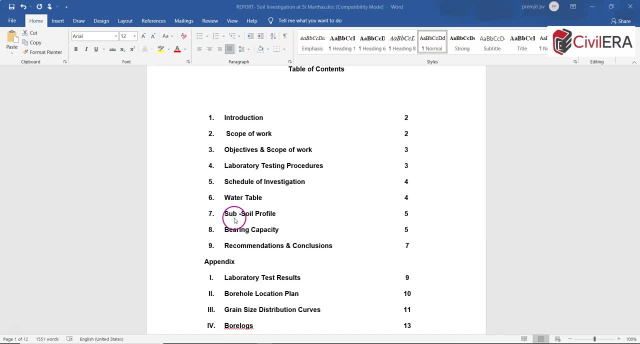 procedures, schedule of investigation, watch table, recommendations and calculations and so on. You can also see an appendix, which is not at all less important- It's as important as the other things, Where you have laboratory test results. you have a borehole location plan shown there. 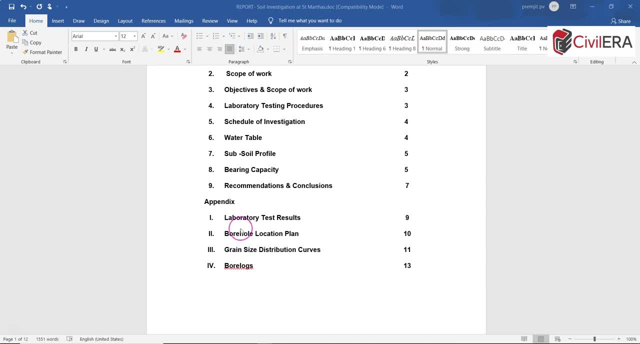 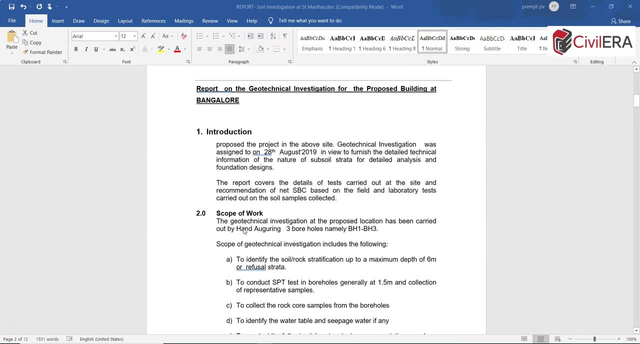 and bore logs. All these are really important and I will quickly take you through these. So in the introduction section it says what the project is, what is the kind of building it is and what kind of scope the consultant has, and it is summarizing that what kind of 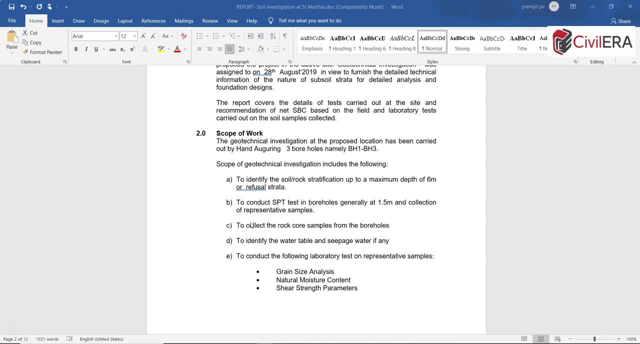 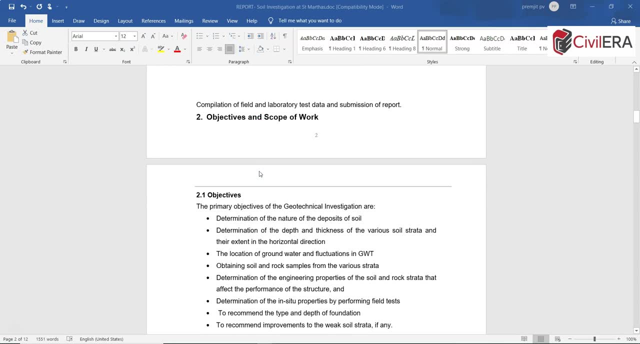 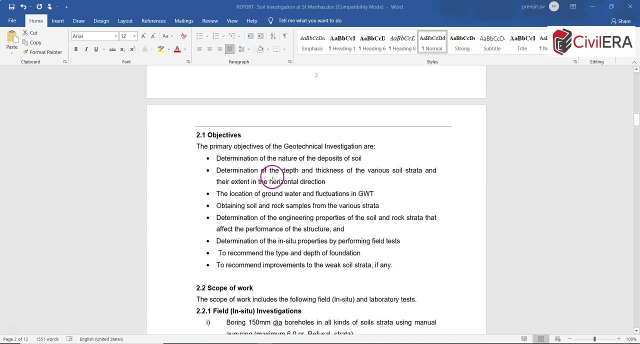 tests are going to be done in this particular report. So that's written here: grain size analysis and various things. Then he is taking you through objectives and scope of work, where it includes something called determination of the nature of the deposit of soil, determination of the depth. 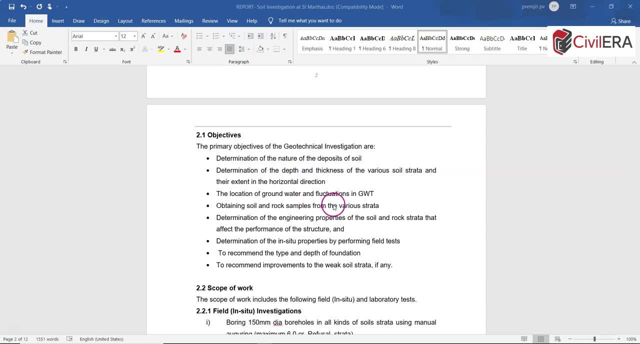 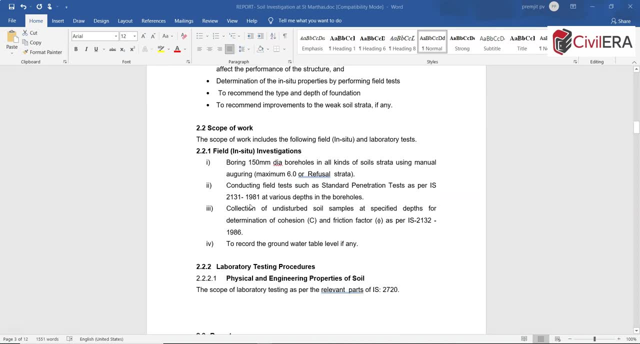 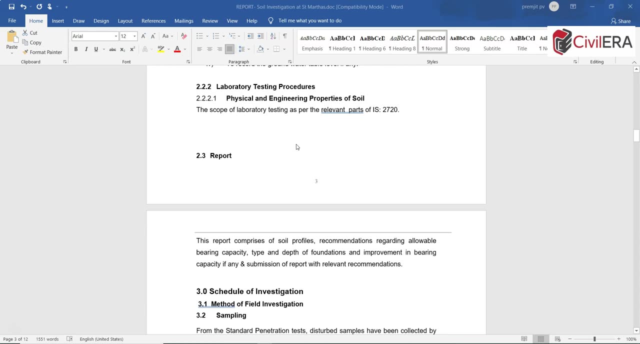 and thickness of various soil strata and so on. So it's directly readable. It gives you every information about the objective. Now, the scope includes investigations, It includes laboratory tests and producing a report. Even that will be clear enough. You can directly read that. 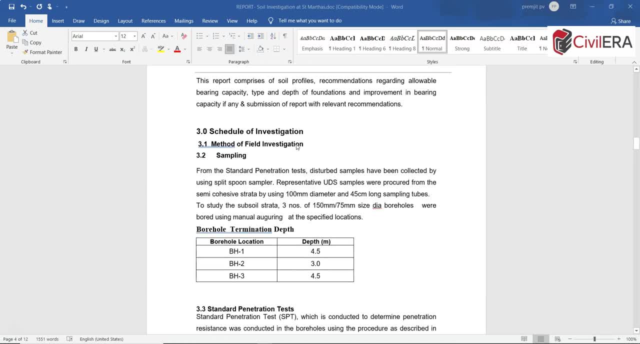 I don't have to. I don't have to spend much time on explaining these. Any soil report. if you get that, you will be able to firm that up In case. if you want this report for reference, you can always write back to me. 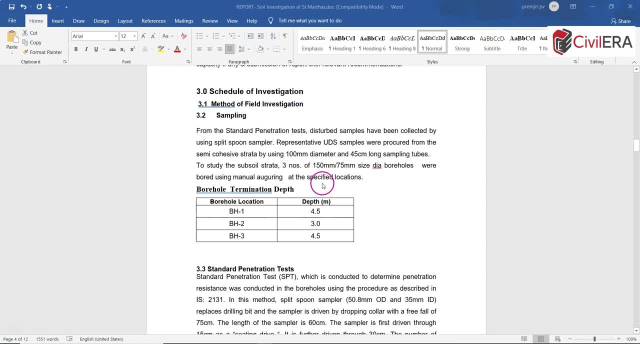 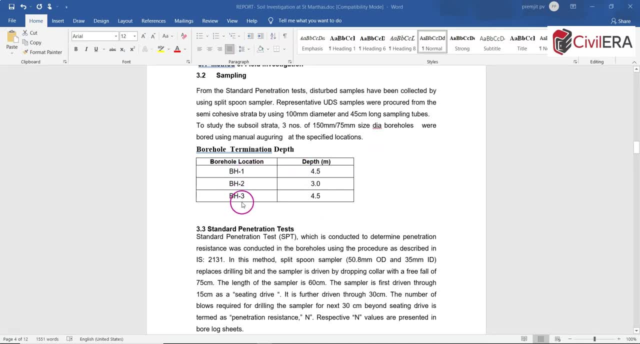 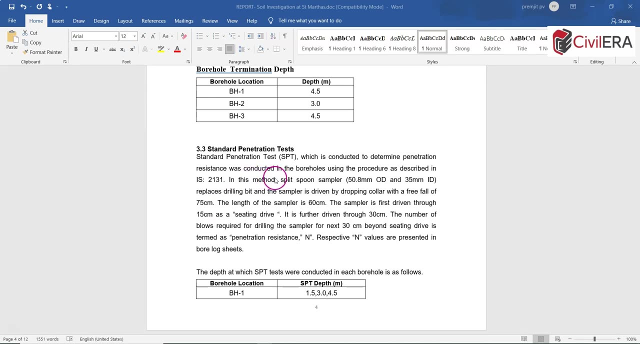 Now section three here explains how the field investigation is carried out. It says how the sampling is done and the borehole depths for each of the holes. Now three. three explains how the SPT is done. It's adhering to IS 2131.. 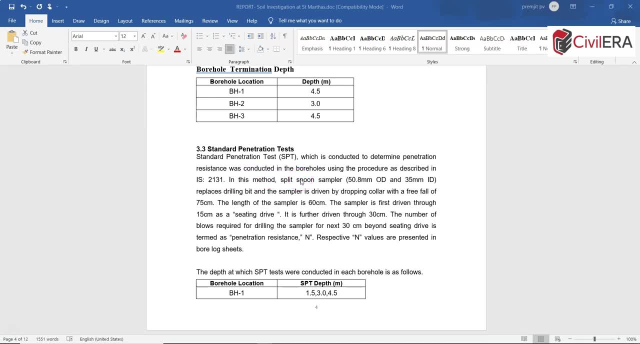 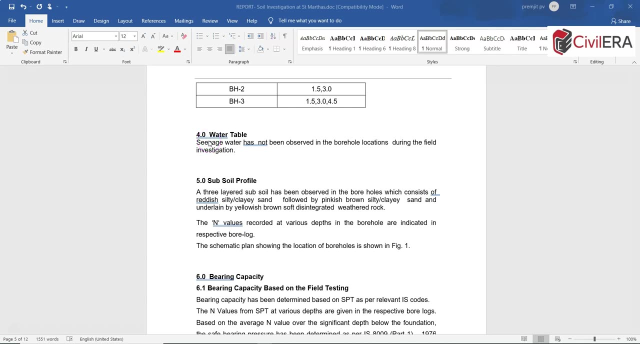 The various aspects are mentioned here which most of you will be aware of. SPT is a very standard test which most of the site and structural and geotechnical engineers are familiar with. Now, in many cases there might be water table and if there is any, it will be reported here. 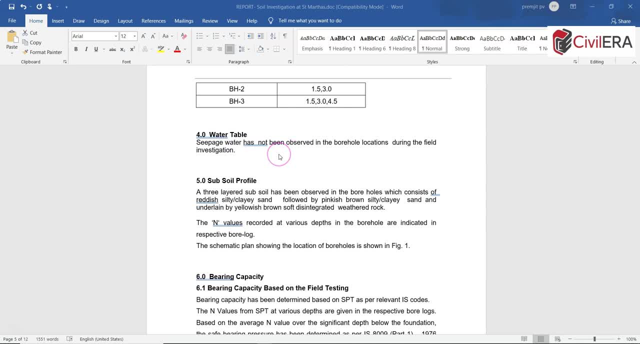 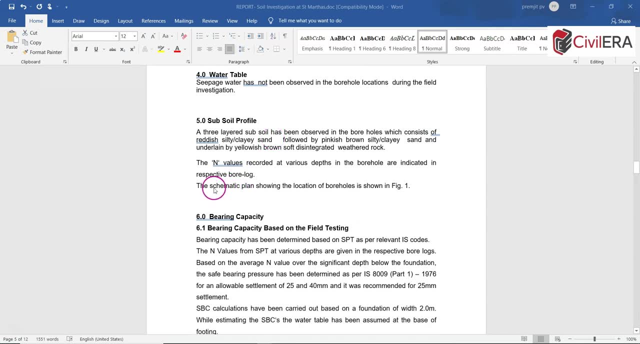 as well. So it says seepage water has not been observed, which means that the water table is not really high. Section five is sub soil profile And there is a reference to a schematic, A schematic plan for the location. all these we are going to see in some time. 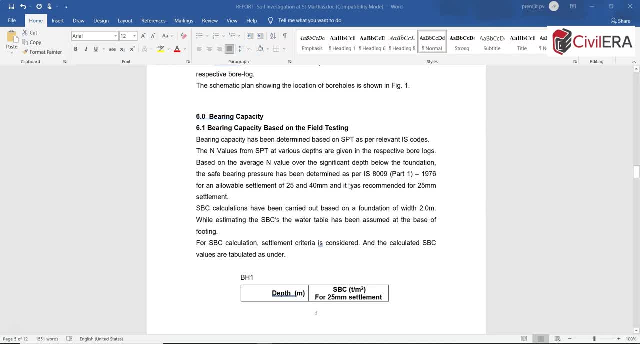 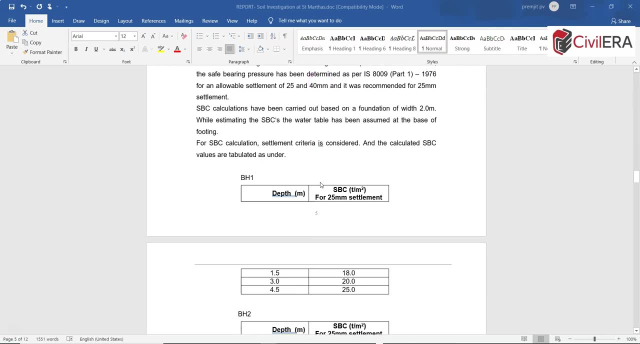 And here there is a summary on the bearing capacity, which is very much needed if it is an isolated footing. And then we have to go through SBC and then size the foundations. So here, at various depths, you are given the SBC for 25 millimeter settlement. 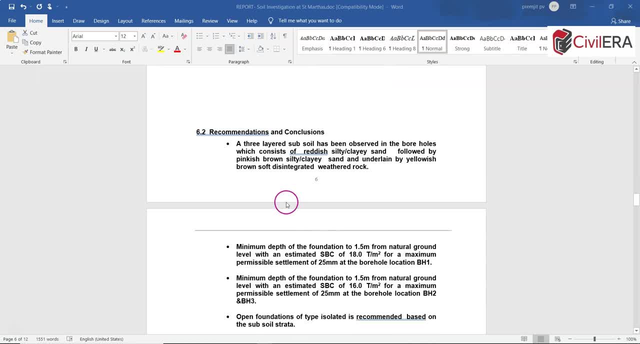 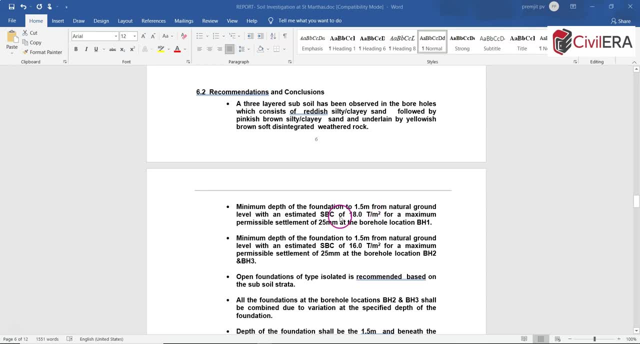 And the section also includes a recommendation and conclusion which says that a three laid sub soil has been observed And it also says the minimum depth of foundation And it also says what can be the SBC there at 1.5 meters. 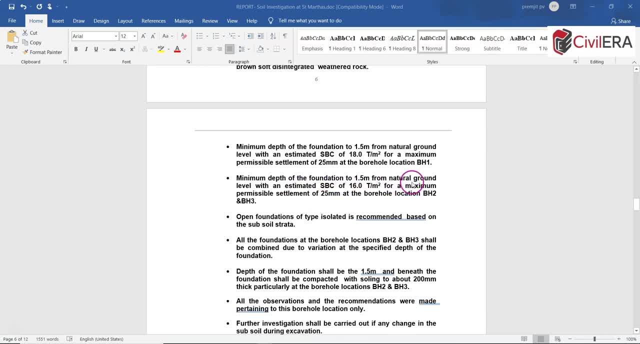 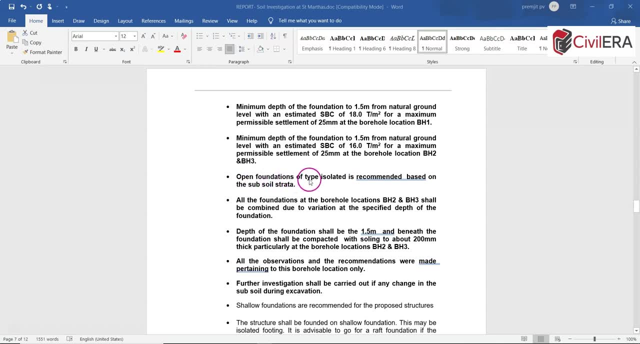 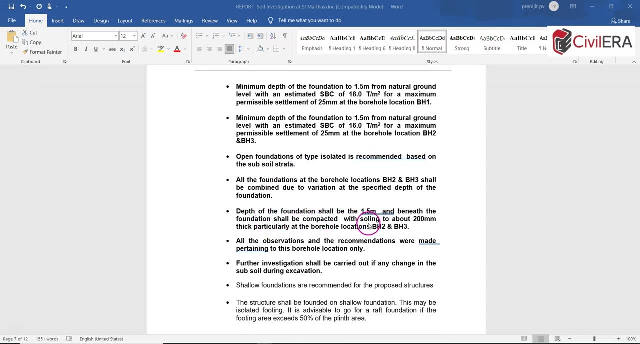 Minimum depth of the foundation from natural ground level for the other boreholes. So all the location values are given And the recommendation is open. foundations of type isolated is recommended based on the soil strata, And here there is a recommendation for providing stalling of about 200 millimeters. 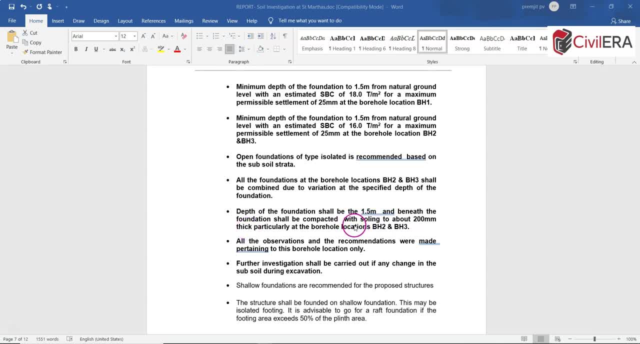 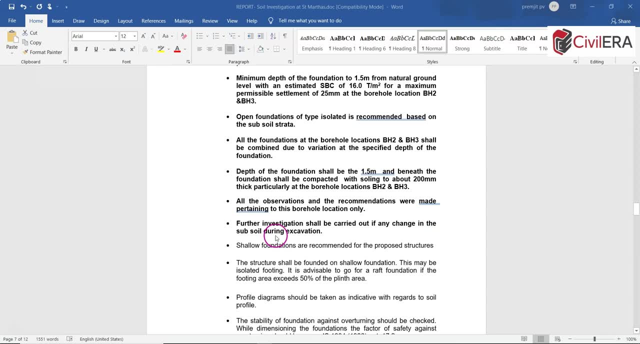 So all these are important. The site needs to execute This. the stalling needs to be provided below the foundation. The consultant also recommends for further investigation in case if there is any variance in the soil strata at site when actual work is executed. 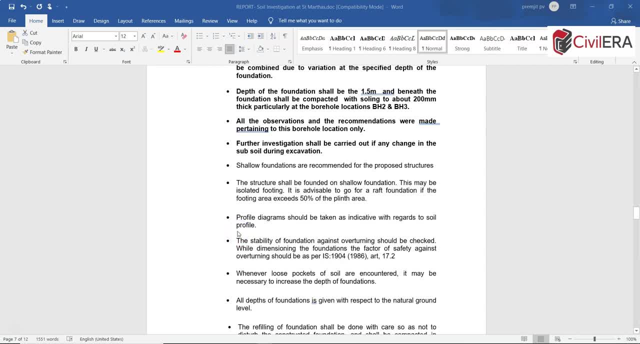 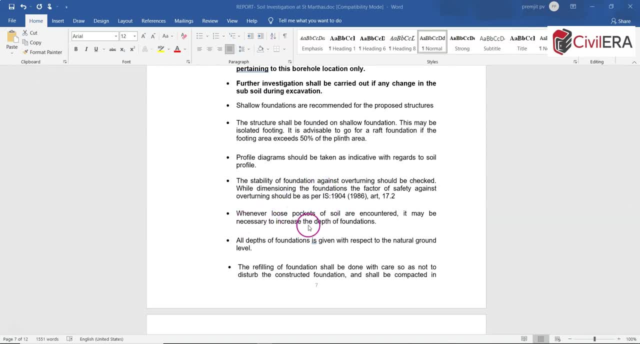 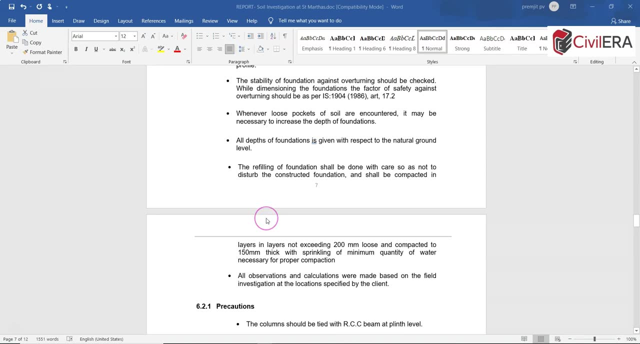 So all these are important to note and do as per this. Now it says the stability of foundation needs to be looked into. wherever there is loose pocket of soil encounter, It may be necessary to increase the depth of foundations, And so on. So all these are to be looked into carefully and then it needs to be adhered to. 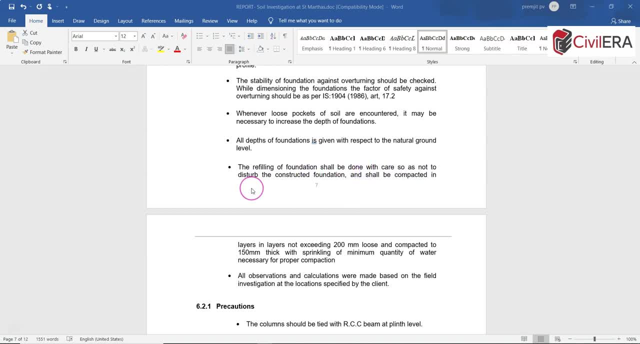 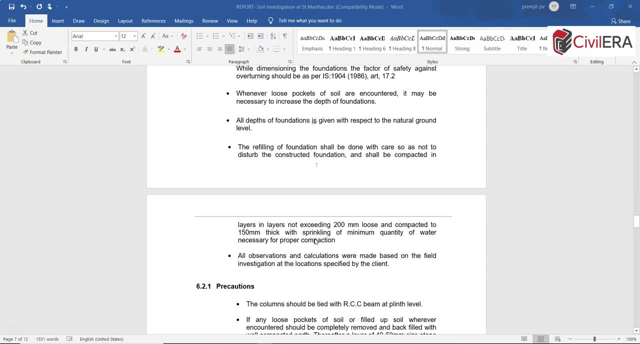 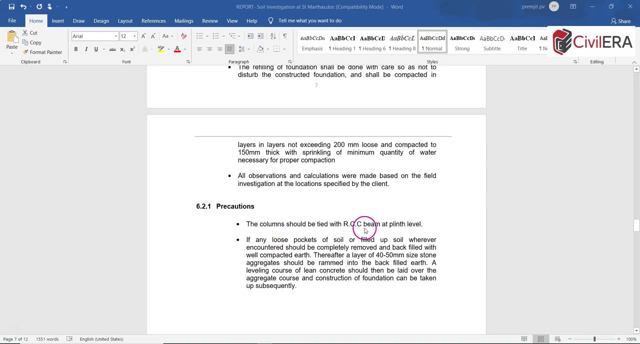 Refilling of foundation shall be done with care so as to not to disturb the constructed foundation and shall be compacted in layers. All these are recommendations and this needs to be stick to, And there are some precautions also mentioned here. The column should be tied with RCC beam at plinth level. 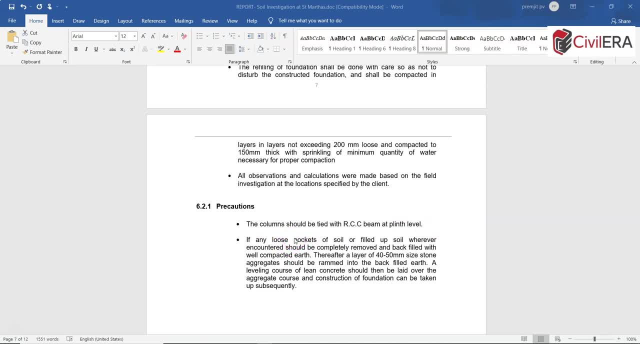 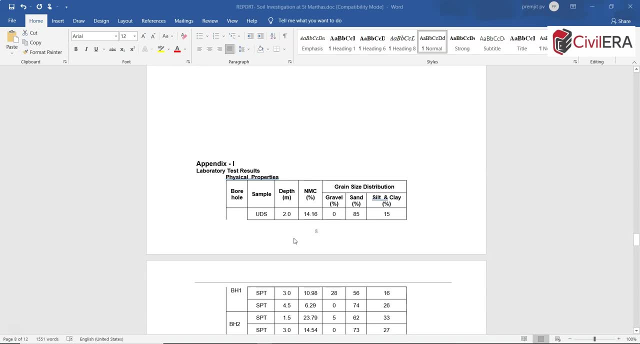 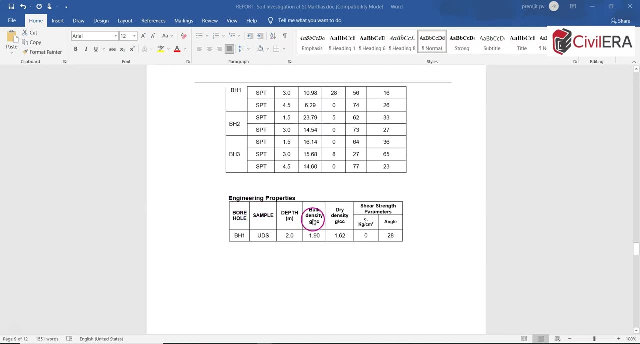 And about the loose pocket. So all these points are to be looked into and then adhere to when we are doing that. So there are appendix here which gives you the laboratory test results. It gives you the grain size distribution, It gives you the engineering properties like shear strength and also bulk hand dry density. 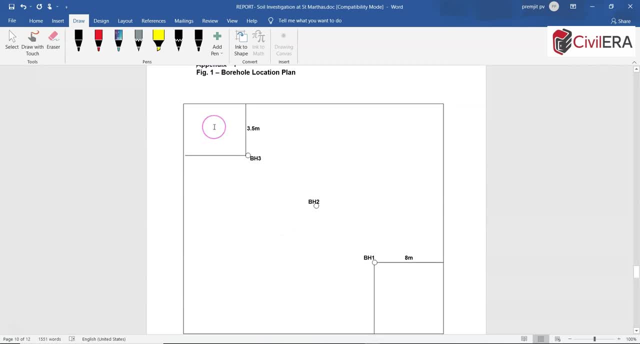 of the soil. And here it shows you the borehole plan, which is very clear. The site is large And there are three boreholes in the site And then there is also an eel and it is in a diagonal manner so that the entire stretch is covered to left and right and also. 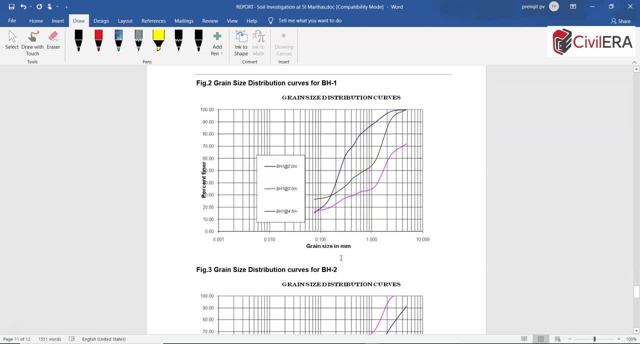 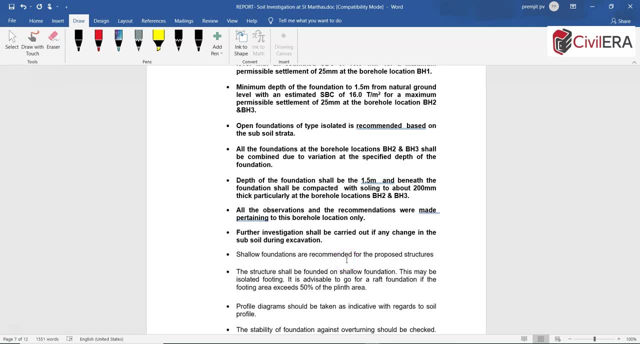 along the leg length and here you have the grain size distribution curves. so this gives you an idea on the profile. so the soil report can be even more elaborate depending upon the importance of the project and the site, and it can contain more information in a more detailed manner. this is: 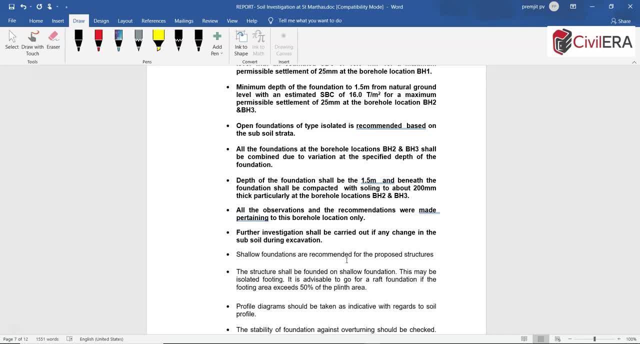 for a mid-scale project in bangalore where the soil conditions are fairly good. so in this manner you can look at the entire soil report and understand the various parameters, including water table and sbc of soil and various things that i just showed you. now i'm going to show. 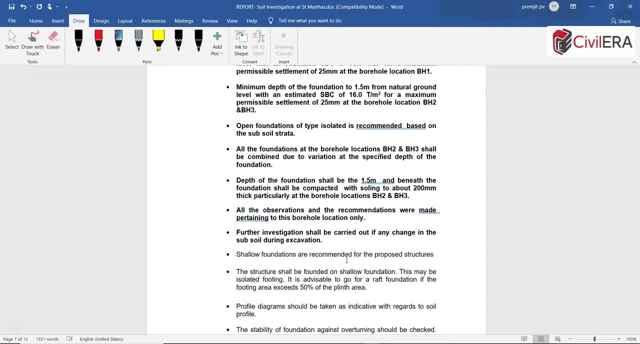 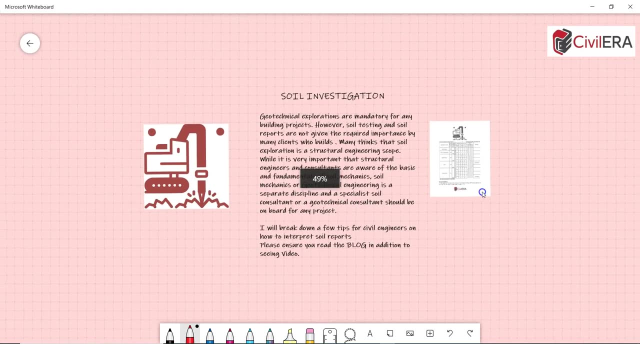 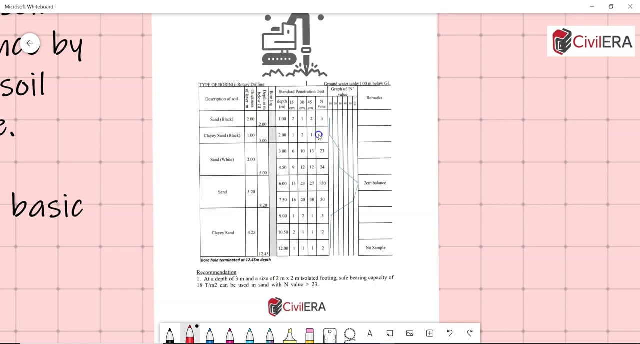 you another soil report which is in a more challenging conditions, which is a compressive soil. so that's where i want to explain a bit more and then tell you what care, what understanding you should have about foundation engineering. so here i have attached yet another soil report here. this time i have shown only a bore log here for explanation, and 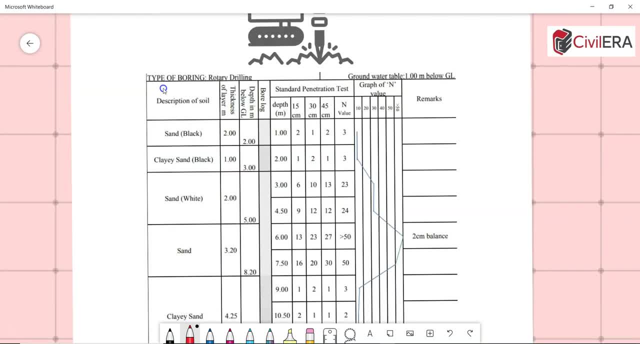 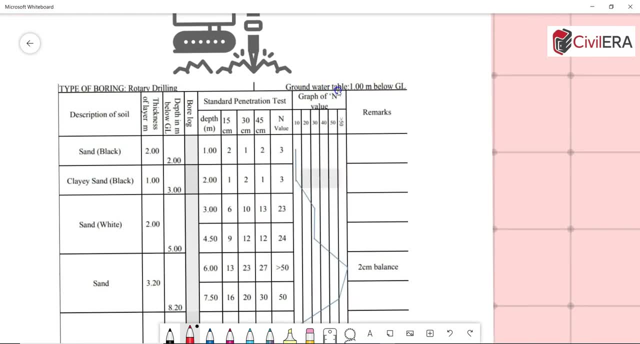 there is a recommendation as well. i have kept so you can see here in this report type of boring, rotary drilling. and then you can see here ground water table one meter below ground level. so there is water at one meter below ground level. next, you can see here the description of the soil: sand, black and 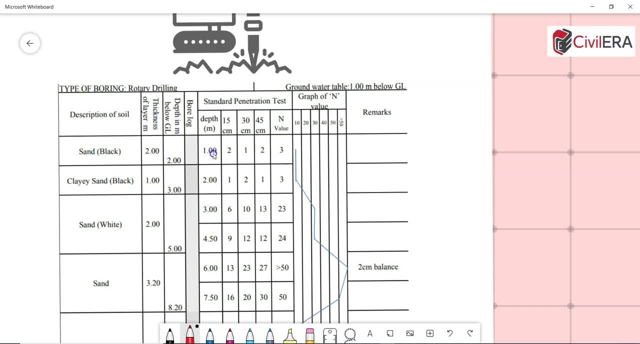 thickness two meter, depth two meter, and here at one meter your n value is three. and at three meter, that is another one meter. two plus one is three. then you have again n value three. so this is very poor soil. and at another two meter that is total five meter. 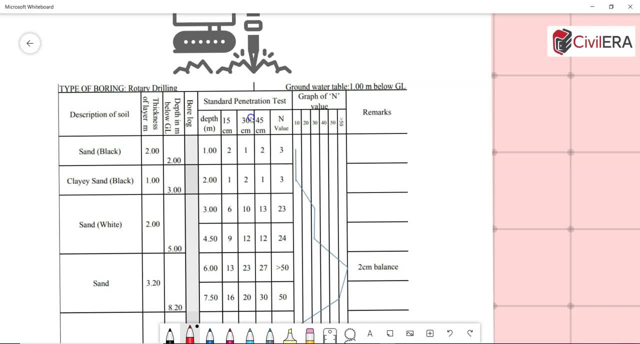 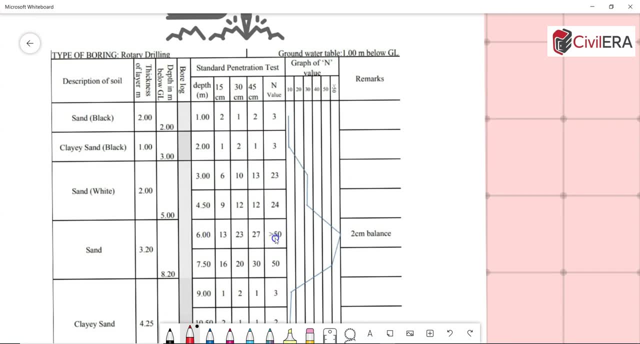 you have 23 to 24 as n value, which is good. now what i want to explain is that as you go down, your n value is increasing, which means your sbc is also increasing. your soil is becoming better as you go down. it's harder as you go down. now, at 8.2 meter, you can. 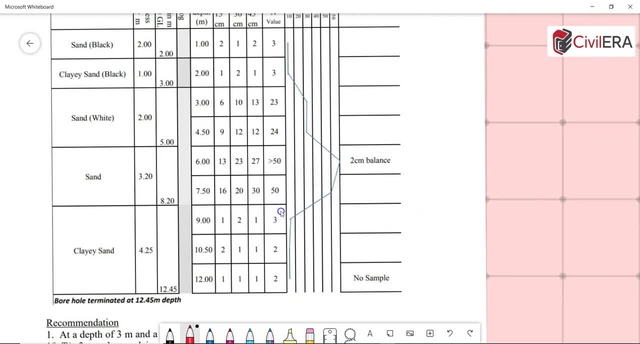 see another behavior where your n value is coming back to three, two and two, which means that you have a very poor clay sand here after 8.2 meters. so this is where you have to be careful, because after a certain height- i think in this case it is after 5.2 meters, that is, 3 plus 2, 5, 5.2 meters you have. 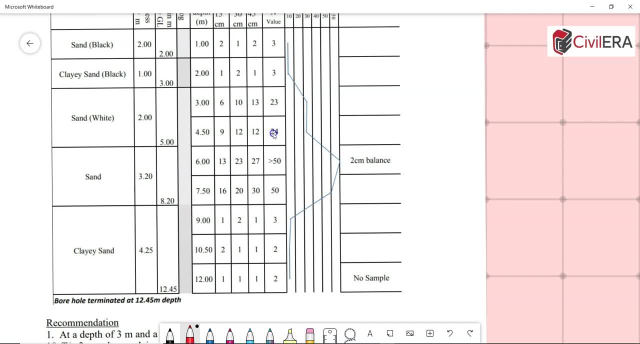 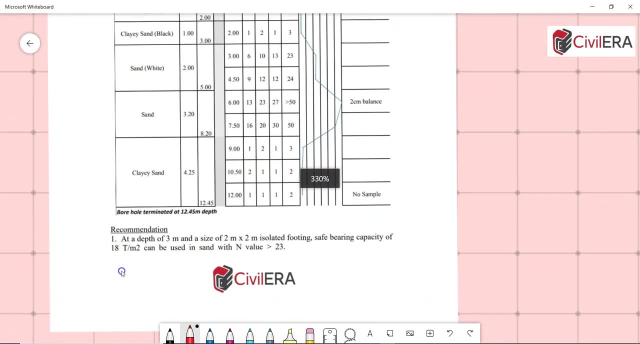 again poor soil and this is where you have probability of compression or settlement. so let us see the recommendation from the consultant in this. at a depth of 3 meter and a size of 2 meter by 2 meter, isolated footing, safe bearing capacity, 18 tons per meter square, can be used in sand with. 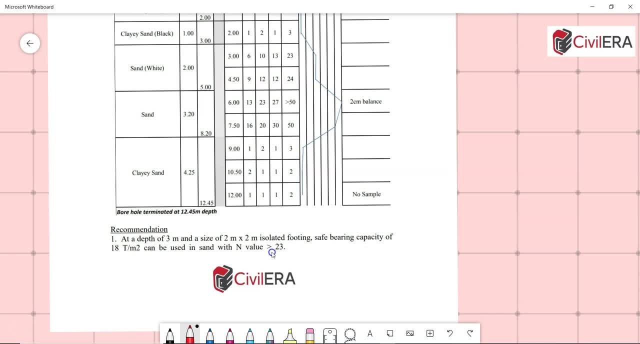 n value greater than 23. so this is the sbc recommendation by the soil consultant. now this needs to be looked at very carefully. 2 meter by 2 meter and 18 tons per meter square. now many you young engineers think like okay, 2 meter by 2 meter is giving 18 tons per meter square and 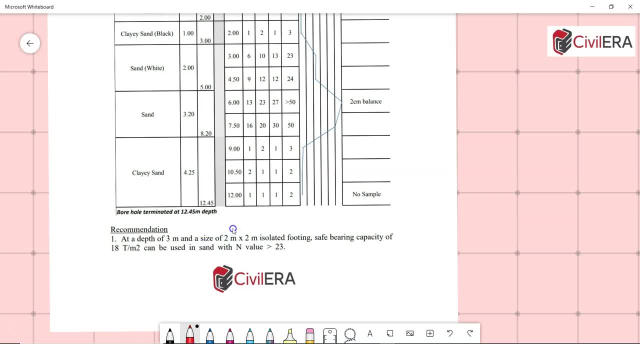 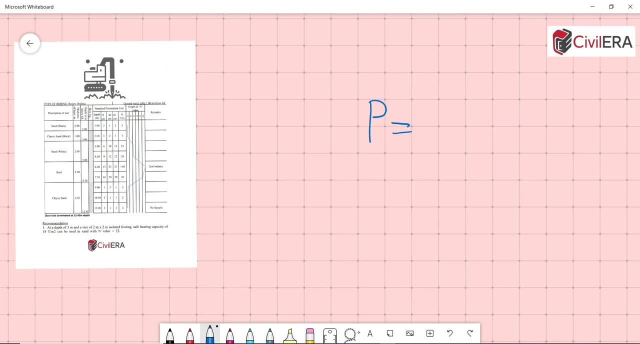 people generally ignore the size given there. this size given there has some significance, which i am going to explain right now. let us consider that we have a load of around 1620 kilonewton on one particular column, and then your sbc, as per the report, is 180 kilonewton per meter square, and 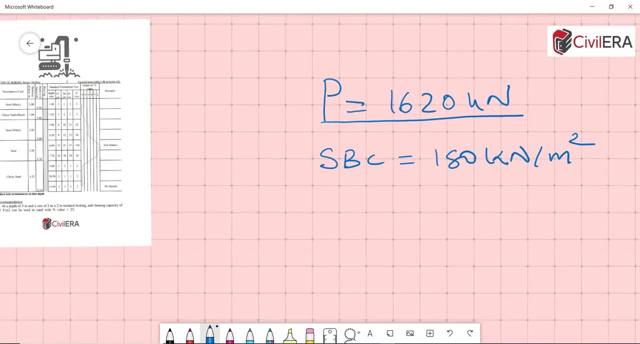 let us consider that this p is inclusive of all the cell seat and everything, and then you need to consider this. so this is the unfactor load. so your area is 1620 divided by 180, which will give you around 9 meter square, and i'm considering the. 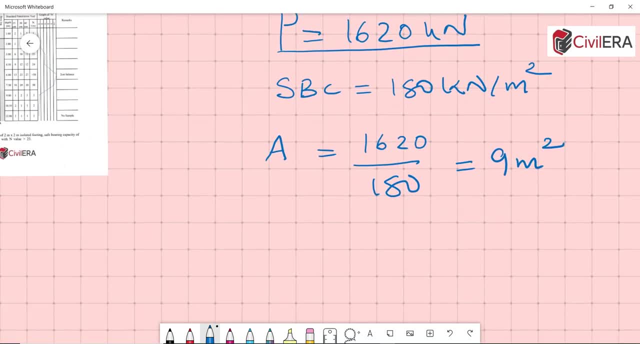 base to be pinned and there are no moments to be taken care of. so let's assume that 9 meter square is needed and if it's a square footing, you will have 3 meter by 3 meter requirement. now the question is: can we give this as a solution? we have met the area requirement. we have taken care of the. 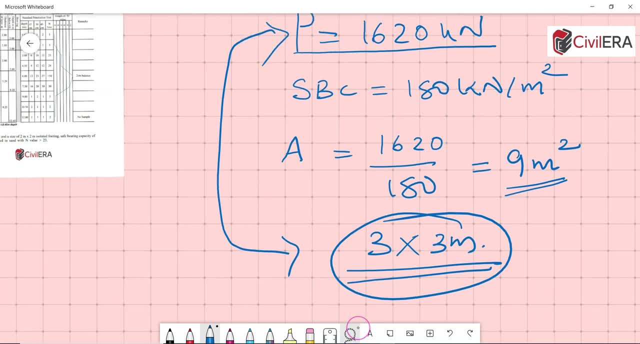 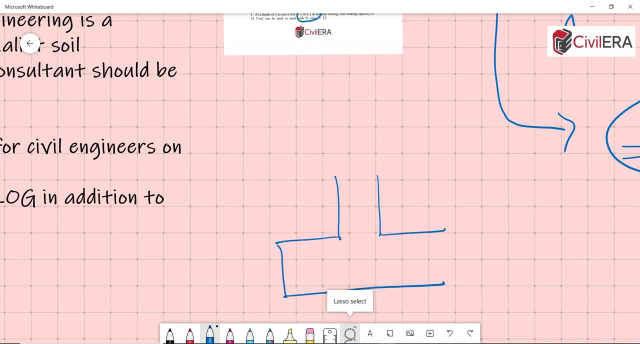 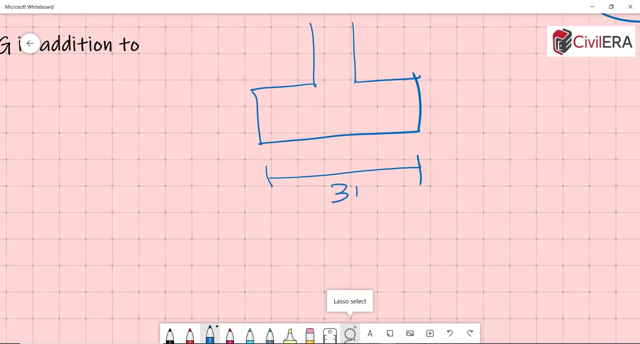 the load. now my question is: can we give three meter by three meter footing? so if you have something like three meter by three meter footing, then approximately the pressure bulb will be around two times that of the width. so if you have this as three meter, it's likely that your pressure 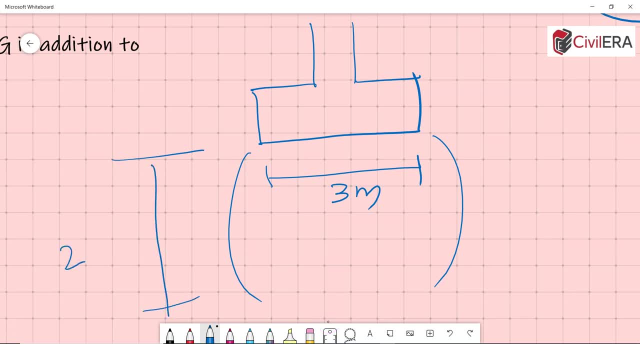 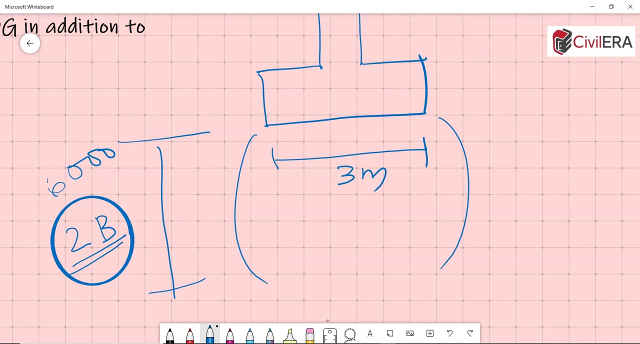 get dissipated at a depth of around two times the width. this is a approximate rule that i am talking, so this 2b could be something like 6000 millimeter or 6 meters, which means that your pressure is dying down only at that depth, which is around 6 meter. now, what is the problem with that? now, if you 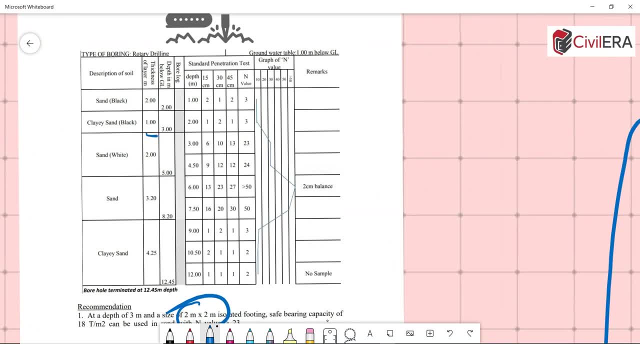 see the report here. if you place your foundation at this level, which is 3 meter from the existing ground level, then your pressure bulb is likely to cross this particular height, which is 5 meter, if you are, if the size of the footing is more than about 2 to 2.5 meters. so that's the reason the consultant 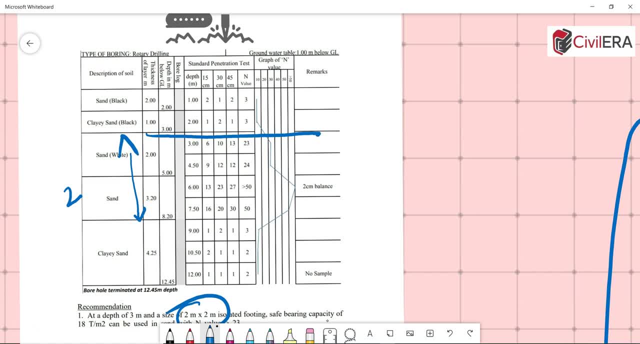 has given the size 2 meter by 2 meter. if your size is more than that, then it is likely that your pressure bulb will get into this area where your end value is very less and the soil is soft and compressible. so if you give three meter by three meter footing, 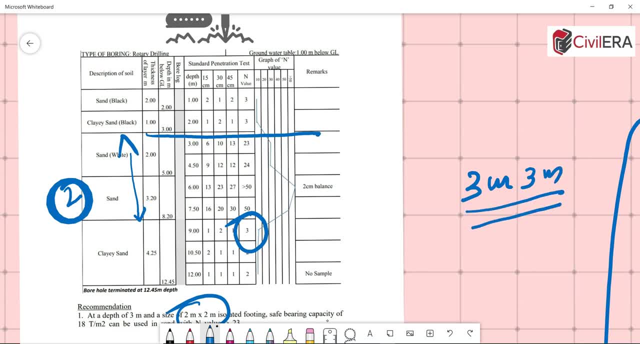 then there are chances that you will have issues with the compressive soil. so that's the reason the width is restricted to two meters. so what you have to do: your scheme needs to be robust. your scheme should account for this and then ensure that your column loads are within. 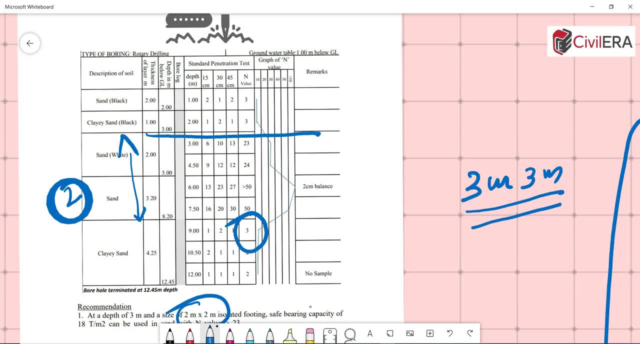 limits. so you might have to arrange your columns, you might have to have number of columns decided based on this particular behavior of soil. you cannot afford to have as much size as you want, even if the footings are not clashing, even if you are not having very close by.